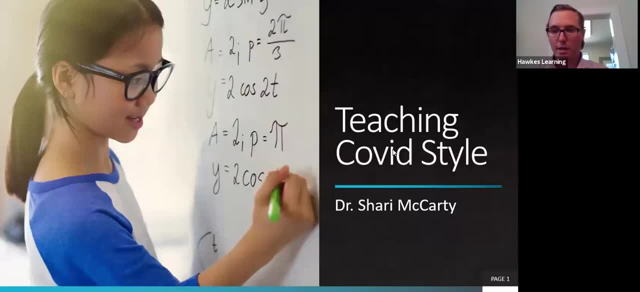 All right, so we're at two o'clock right now, so I think we're going to go ahead and get started with today's webinar. First and foremost, thank you everyone for attending today. My name is Brian Dunn. on my work at Hawks, I'll be kind of hosting this webinar and we are very happy to share and 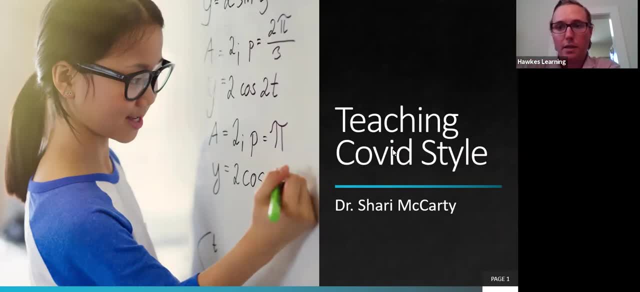 welcome Dr McCarty for her teaching COVID-style webinar today. She's going to go through her teaching COVID-style webinar and towards the end, well, obviously you guys are going to see a little Q&A option. if you want to ask any questions, We're going to answer the questions towards the. 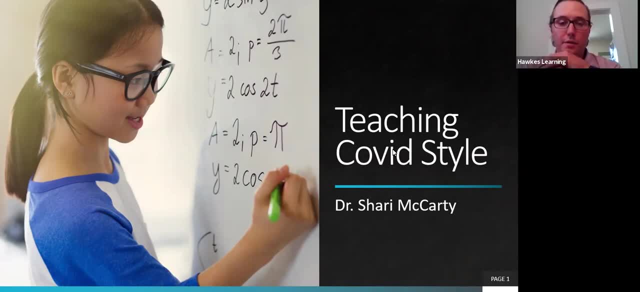 end of this webinar series today, so feel free to ask any of those questions in that Q&A, and Dr McCarty or myself, if it's a Hawks-related question, we'll be happy to answer anything. So, Dr McCarty, it's all you. Thank you. Well, welcome everybody. You're actually learning. 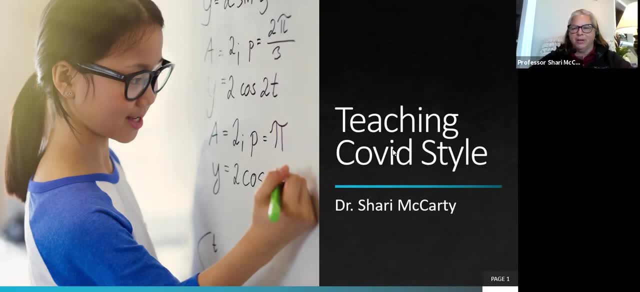 about this from my list. I'm going to start off by talking about teaching COVID-style, which I'm sure no one has not heard of COVID, so we're not going to get into that, but we're going to go ahead and get started. of what? 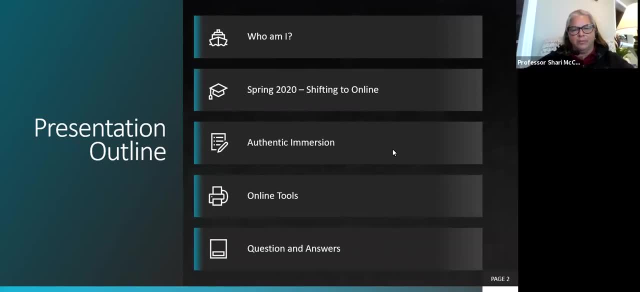 the webinar today will look like. We'll start out talking a little bit about the COVID-style and a little bit about who I am in the background. the spring from 2020, and how it shifted very quickly from face-to-face to online. also including what we're doing. fall of 2020, and how 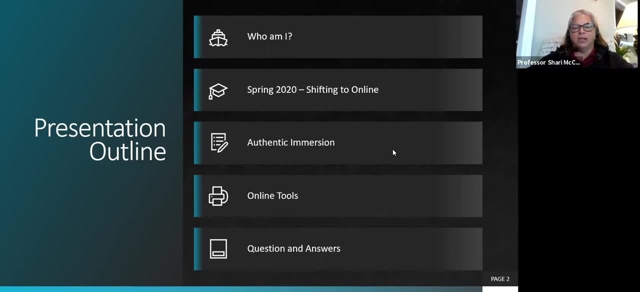 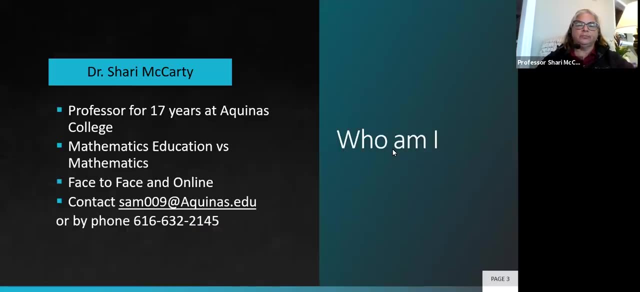 we're trying to have an authentic immersion in the classrooms, some online tools that I've found useful, and then certainly plenty of time for question and answers at the end. So, first of all, who am I? So I have been a professor at Aquinas College and Aquinas College. 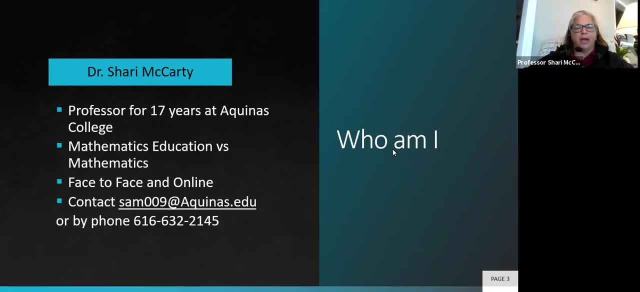 is a small liberal arts Catholic college located in Grand Rapids, Michigan, and I'm a one-person math education department. I'm housed within the Department of Mathematics. However, if you're not clear on the difference, math educators work on helping students learn about how other students 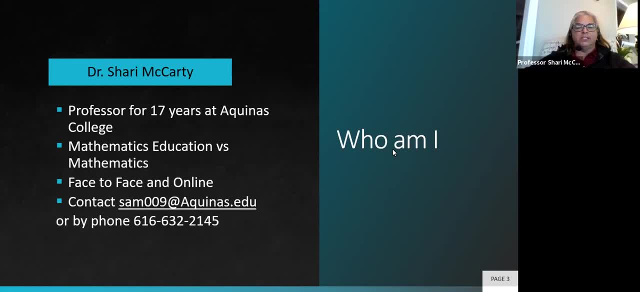 learn mathematics and how to teach mathematics versus specifically mathematical content. So our math education program has three courses, And two of them are content related, where the pre-service teachers are reviewing content from K to 8, and then we have a methods course in which we learn to enact those lessons and what that 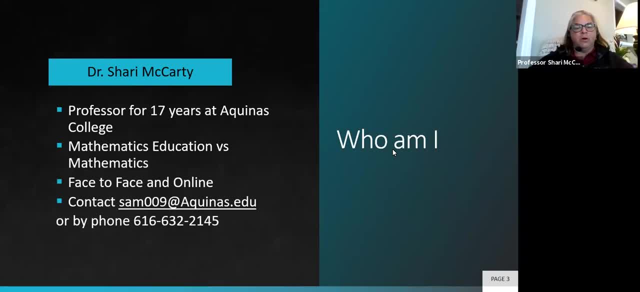 might look like in front of students. So I teach both face-to-face and online regularly, although my online courses have been general education courses in algebra and math for liberal arts. So shifting to online math education courses was definitely a challenge, But I'm here to share some of my learning experiences and some of the things that may be. 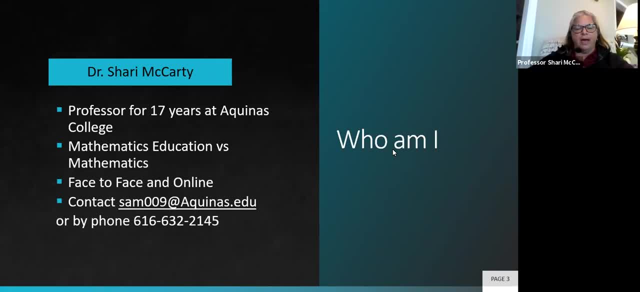 beneficial to you if you're looking to work in the future. I'm very excited to share my full-time thesis project with the University of Los Angeles College of Science and Technology, And my content is also available on the Office of accountability and accountability with the. 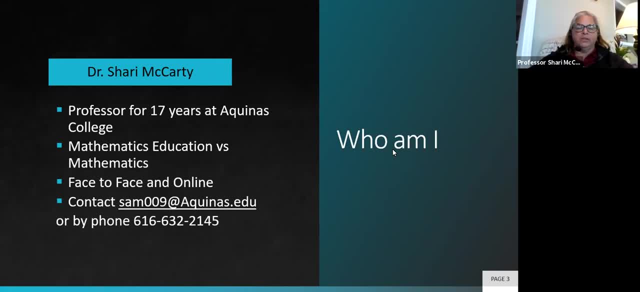 University of Los Angeles College of Mathematics, So I'm excited to share this with you. My question is: what are your vulnerabilities? So if you're looking to learn math in high school, how do you deal with those? So, if you're looking to learn math in high school, how do you deal with those? 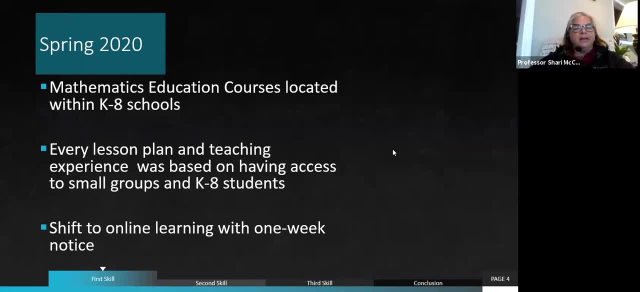 What are your vulnerabilities? So let's think back to spring of 2020.. March, in particular, we had well prior to that. let's start back in January, where our classes started within the K-8 schools. So the Aquinas College courses took place on the campuses of other schools, where we had our own dedicated. 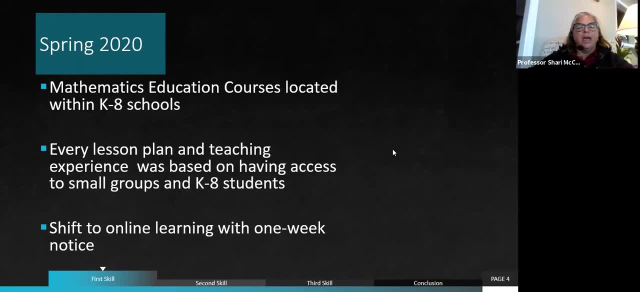 classroom for my lectures and the students learning, And then during our class time we also were able to go into an actual classroom and either tutor in small groups or take over classrooms for the teachers and lead the students in math instruction. So every lesson plan and 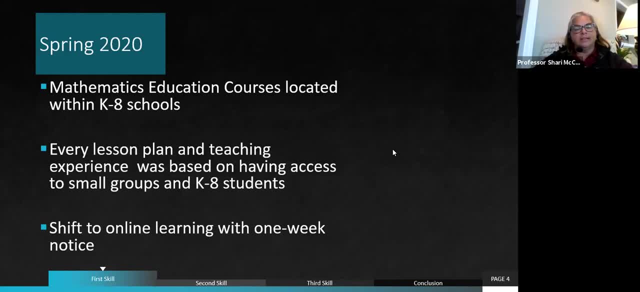 teaching experience that I had developed over the last 16 years was based on having access to real live students, having that authentic experience where our pre-service teachers could use their improv skills Not knowing what their little students were going to ask them. Also, practice using their 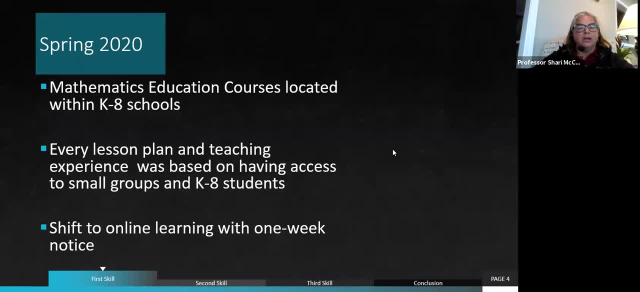 vocabulary and methods that we had been talking about in the classroom and reading about in our texts, And so it was a wonderful experience. The classroom teachers appreciated having the extra help and some new ideas, So we were able to help their students and we were also able to gain the 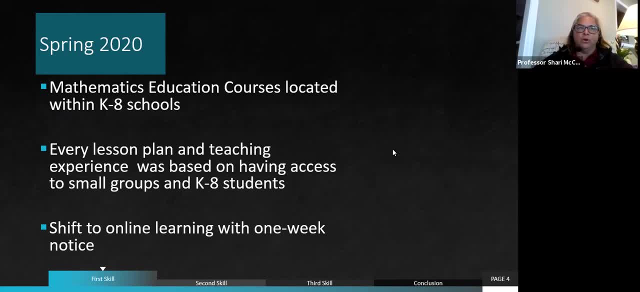 valuable experience, So it was definitely a win-win. We had one course that was situated in more of an urban school setting and one course that was situated in a private school setting, So they were different settings. So the students get to experience that as well as just have the. 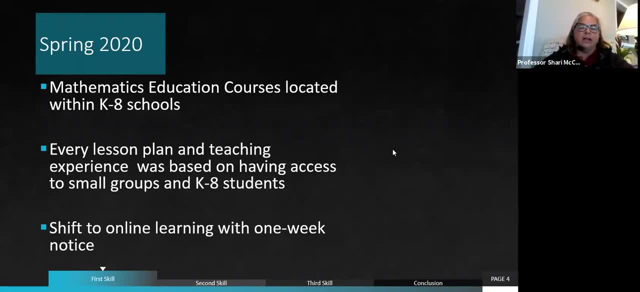 opportunity to be in the classroom, see what it takes for an elementary teacher to schedule their day and the challenges of interruptions. So we leave on our spring break in March of 2020.. And at the end of spring break we receive an email from the president of the college stating that we were going to have one additional week of 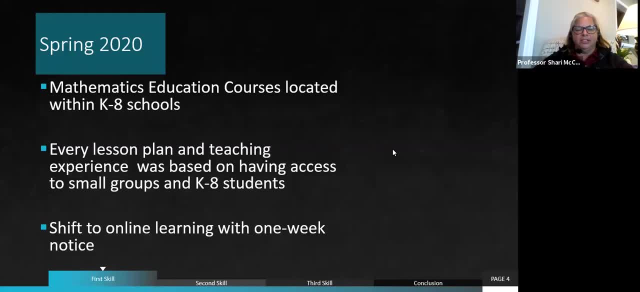 spring break to prepare ourselves and our students to transition to 100% online. So in one week all faculty and students were transitioning from what has been an ultimately almost entirely face-to-face college to an online learning experience, And for me we were out of the K-12 classrooms, K-8. 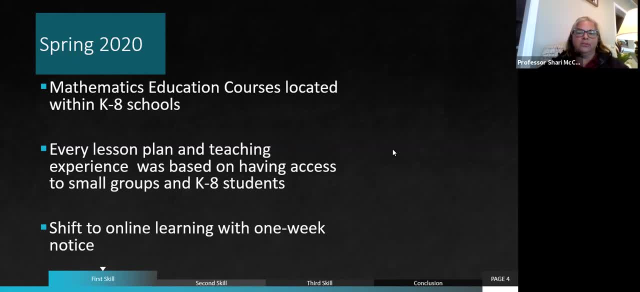 classrooms And I was struggling with trying to think about what I was going to do in the spring break And I was struggling with trying to think about how can I reenact and give these students the same authentic experiences. So we shift to online learning with one week's notice. 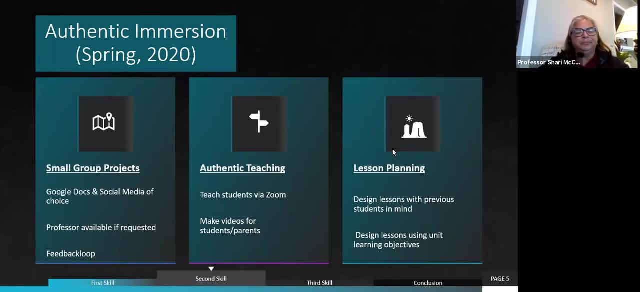 So what were some of the things that I had? I came up with quickly. Well, when we were in the Aquinas classroom, we did a lot of small group projects, So during that we were gathered around tables, we were having discussions. I was available to pop in. 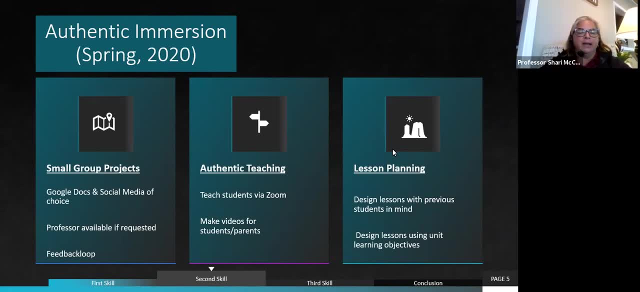 and out of groups. but I would no longer be able to do that, So I shifted to an idea of using a Google Doc, in which the small groups could collaborate simultaneously And they were allowed to use a social media of their choice. So some students used Facebook, some students used 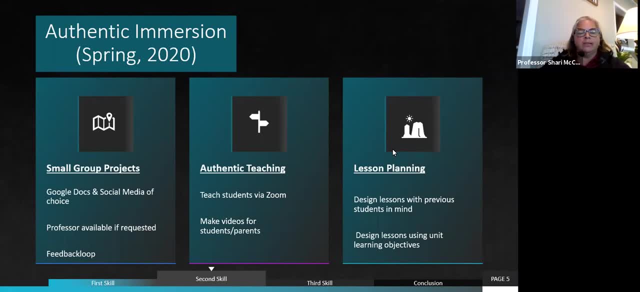 FaceTime, Zoom, Skype, anything that they felt comfortable in- and they collaborated on a Google Doc simultaneously. I was available to them if they would like me to join their small group, but I was not hovering in each group because they were. they were meeting at times that were convenient for them, so while I 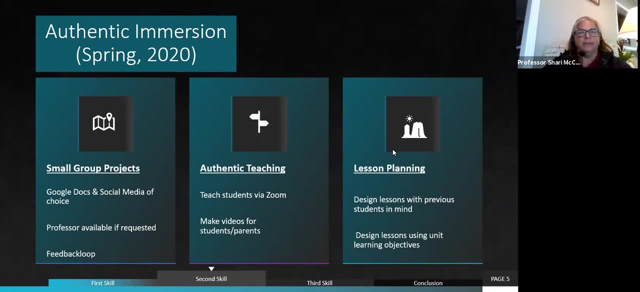 say simultaneously they were not using their class time. their group of four students just had to pick a time that would work for all of them, and then I looked at the Google Doc and provided feedback before the next class session. so that was our feedback loop. the challenge of authentic teaching became. 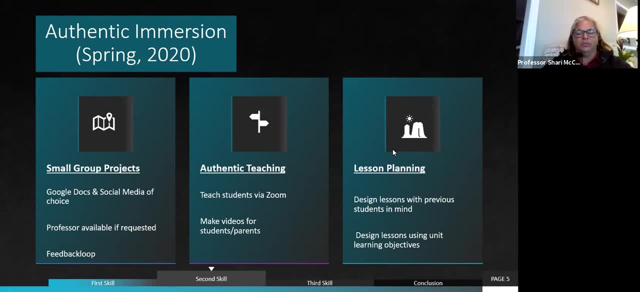 real. the students in our k8 classrooms were transitioning themselves and students were not as familiar at that age- nor were their parents- with zoom meetings and Google classroom and things of that nature, so we lost our direct access to students. at that point, the schools felt like it was just too. 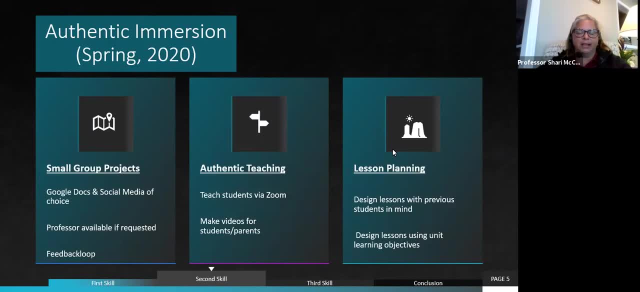 overwhelming to have us joining in or participating at that level. so my teachers- pre-service teachers- then had to just seek out student volunteers, relatives, young sisters, brothers, cousins, anybody. they could. in fact, one student has student volunteers- relatives, young sisters, brothers, cousins, anybody, they said. struggled so much, she set up a zoom session with stuffed animals and acted. 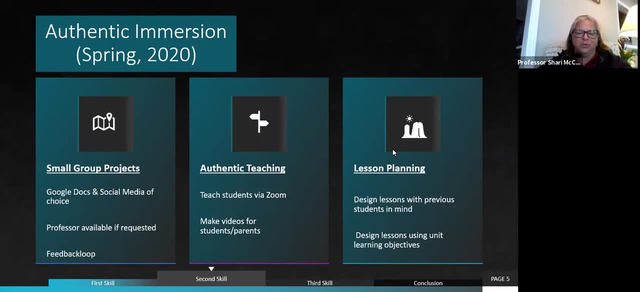 both as the student and as the teacher to submit her project and I certainly gave her credit for the creativity and thinking. what the students would be thinking was actually kind of interesting and worked out okay. so our teachers and the spring were just using zoom with any volunteers they could to 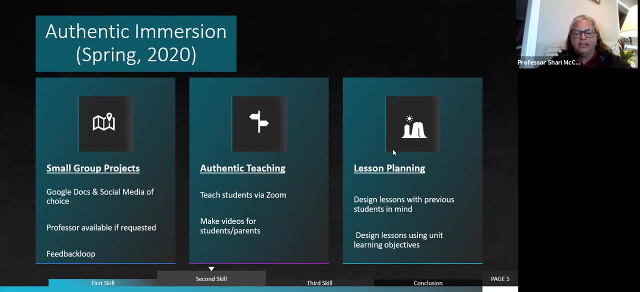 practice their lessons that they came up with they. in addition, I decided to have them make videos for parents and students about math content, so, since the students were not live, I was able to have them create videos on a topic that would be appropriate for students and parents. 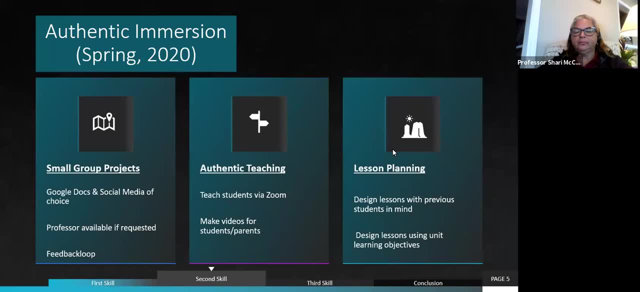 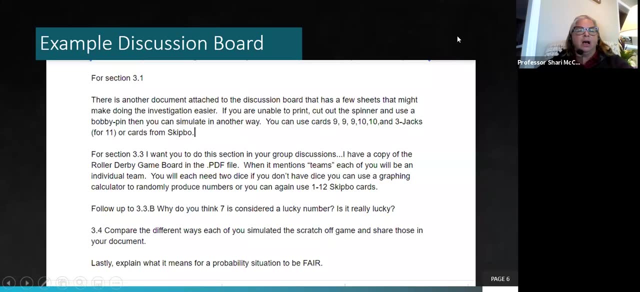 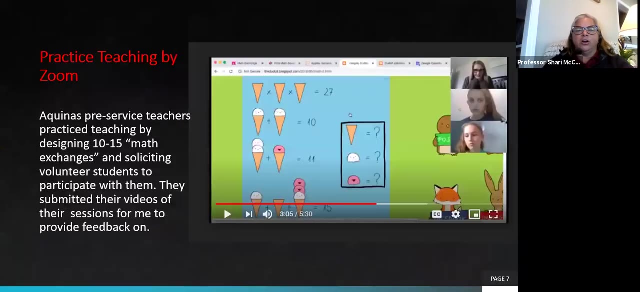 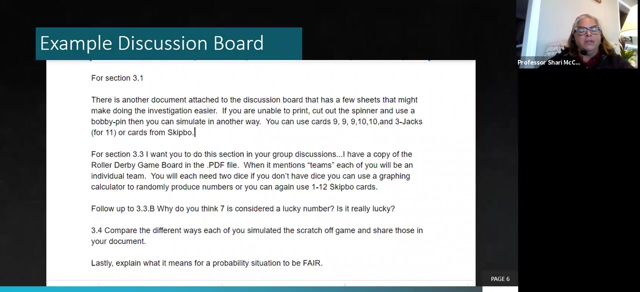 to review at home and hopefully pick up the information. so when we started designing our lesson plans, we ended up thinking about: oops, sorry, I clicked way ahead, I'm gonna go back. so we we started thinking about how we could design lessons and what those might look like. so one of the examples of my discussion boards for 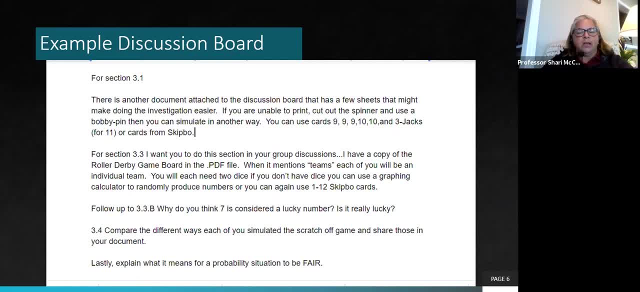 my own lessons would be. this example of using probability and what this might look like in the classroom would be: we would have spinners. the students and the pre-service teachers would be creating a data set and deciding why seven is oftentimes considered a lucky number- and is it really lucky? and I'd be prompting. 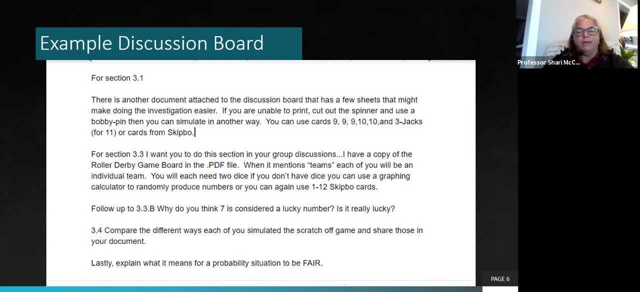 them and pushing them on this conversation. however, when they were in their own groups, they may or may not have access to spinners- they could. they were given one that they could cut out and use a bobby pin. they were also encouraged to use other things that might simulate this. they could use cards. 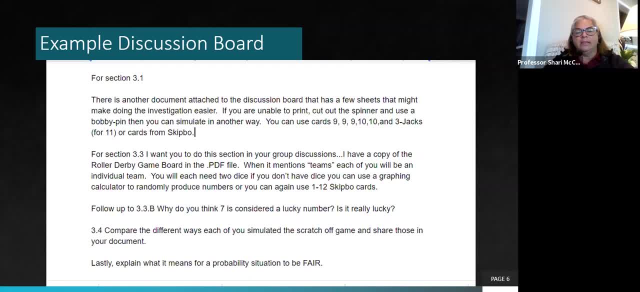 they could use cards from the game skip bow, anything like that. so part of our struggle with learning online was having the students who went home abruptly have materials that they could use that we typically don't know how to use but we typically had available to them in the classroom. so with that challenge like 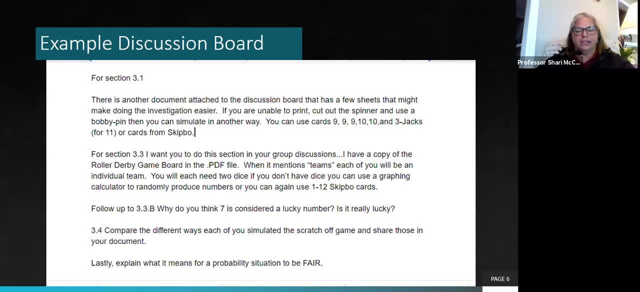 that was great as future teachers to have them think about other things that they could use. so questions like a seven lucky, why or why not, and what does it take to make probability a fair situation. so the the students would think about this in their small group. type their response. I would read their. 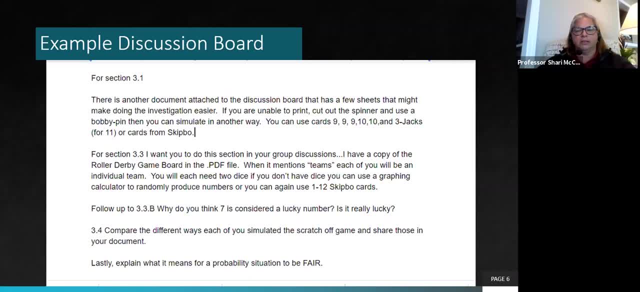 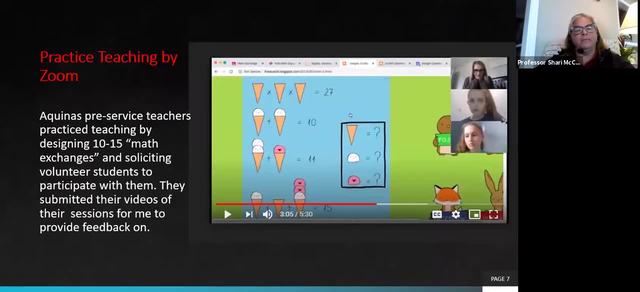 Google document and give them the feedback that was discussed. so that's a type of lesson that we're going to be talking about in the next few minutes. so thank you so much for watching and I'll see you in the next one. I developed a type of lesson that a student might develop was using what we 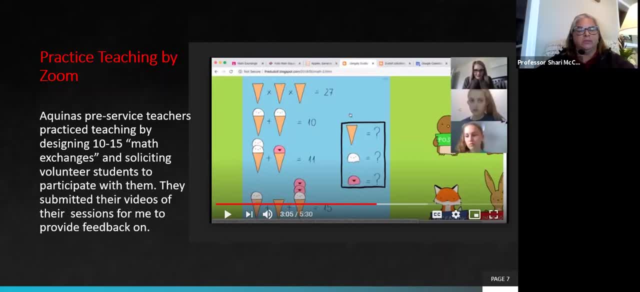 call math exchanges. math exchanges is a specific type of conversation where teacher and a student really work on allowing the student to come to their own conclusions and particularly be able to communicate, so communicate both verbally, in writing and journals or whatever. so this is the screen of a 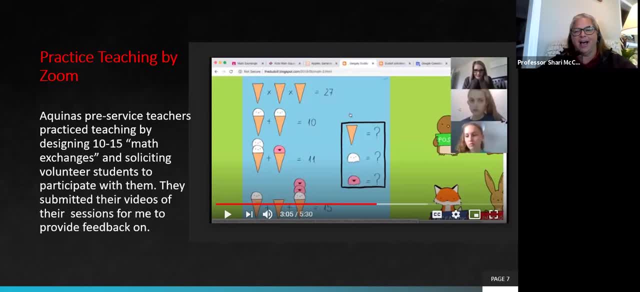 student and her student's course student and her, my student at the top, which is a pre-service teacher, and her volunteer students, who actually happen to be relatives of hers, and she posed this question to them, allowed them to talk with amongst themselves and then she would interject when she was all done. she uploaded this. 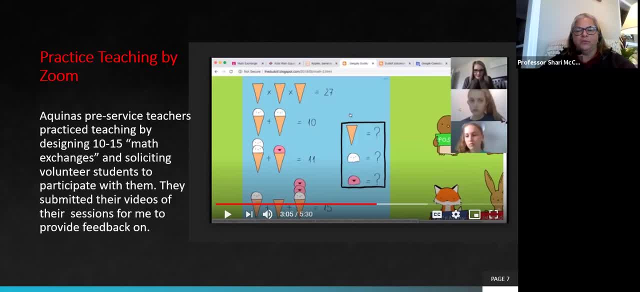 video for me to provide feedback, and it was wonderful because I could stop and show her how quickly she jumped in to respond, how it she didn't allow any downtime for her students to think and talk with one another. she jumped in. she was eager to rescue, which is what I find quite 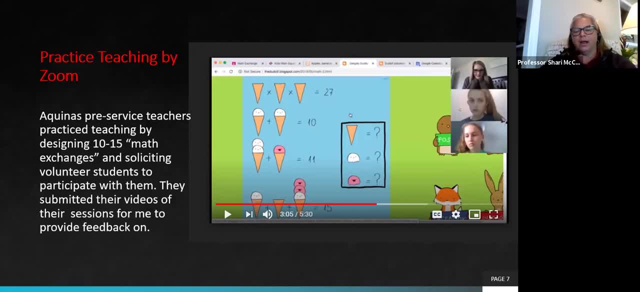 often with my pre-service teachers. they go into this field because they want to help students. they want to help them succeed. so they oftentimes jump in a little bit too soon to interrupt the students thinking: so this was what we worked on in spring. in the fall, 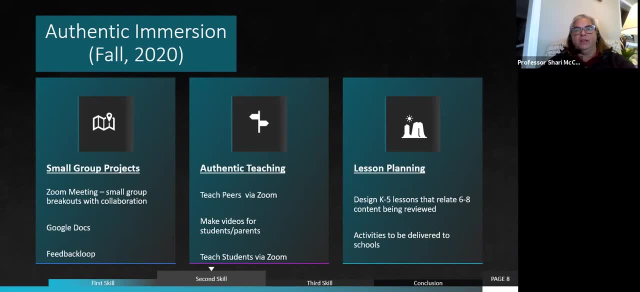 we as in the fall, meaning we started August 19th. so while it's officially not fall by the calendar, we have started fall semester. so August 19th we were trying to think of what could we do to have an authentic immersion. many of our local Michigan K-12 schools did not know, even on August 19th, how 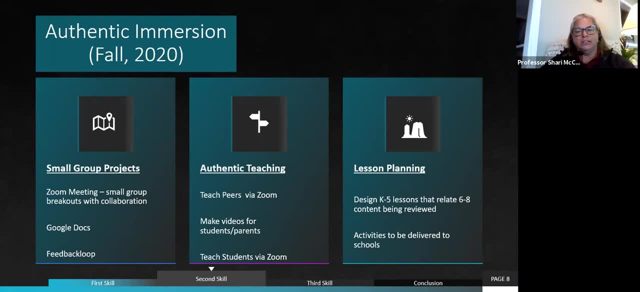 they were going to present their fall to their students. some were starting with completely online families and some were starting with completely online families and some were starting with. some were starting with completely online families and some were starting with completely online for nine weeks and then going to make a decision. some were shifting to two weeks online and then 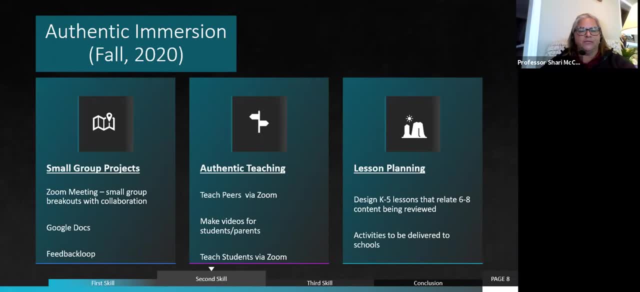 classroom face-to-face. some started face-to-face but rotated days with groups of students, and the days that they were not allowed in school they were to be doing online learning, kind of a hybrid, with Wednesday being a disinfect day. we have a wide variety around us in Grand Rapids of how. 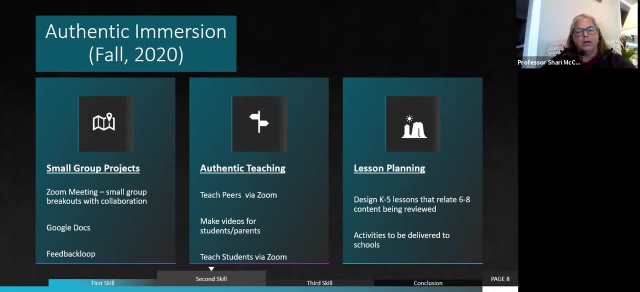 they were going to enter the classroom with. that said, I think we're going to go ahead and wrap up with that said, I think we're going to go ahead and wrap up with that said. I think we're going to go ahead and wrap up with. that being said, teachers were overwhelmed in. 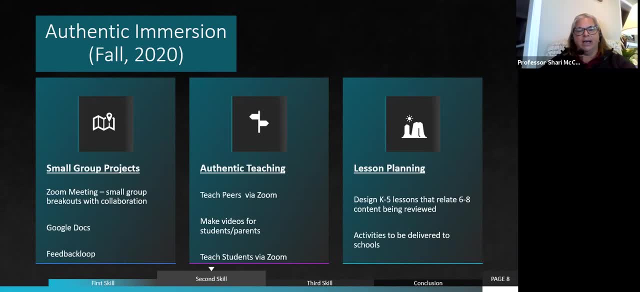 with that being said, teachers were overwhelmed in. with that being said, teachers were overwhelmed in their own preparation for their teaching and their own preparation for their teaching and their own preparation for their teaching. and we're not sure how our Aquinas class could. we're not sure how our Aquinas class could. 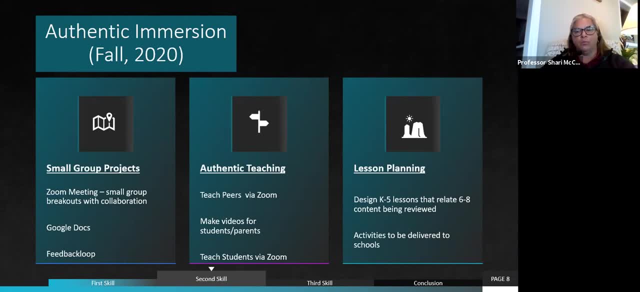 we're not sure how our Aquinas class could integrate with that without causing integrate with that, without causing integrate with that, without causing perhaps more work, more confusion, more, perhaps more work, more confusion, more, perhaps, more work, more confusion, more technology issues and things like that. so technology issues and things like that. so. 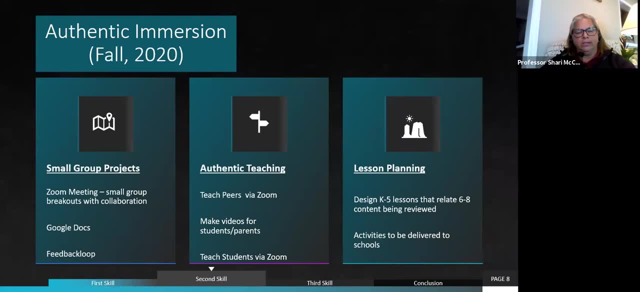 technology issues and things like that. so we ended up working with just one school. we ended up working with just one school. we ended up working with just one school and we are able to do some authentic and we are able to do some authentic and we are able to do some authentic teaching with that school. again, I always 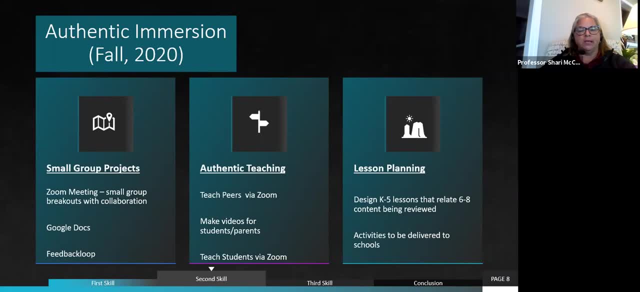 teaching with that school again. I always teaching with that school again. I always teach in small groups. so it was really teach in small groups. so it was really teach in small groups. so it was really important for me to come up with a way. important for me to come up with a way. 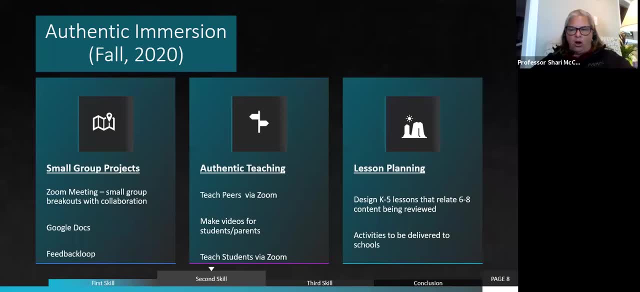 important for me to come up with a way to do small group projects. this time our to do small group projects. this time our to do small group projects. this time our college allowed us to do sima. synchronous college allowed us to do sima. synchronous college allowed us to do sima synchronous learning, or simultaneous learning through. 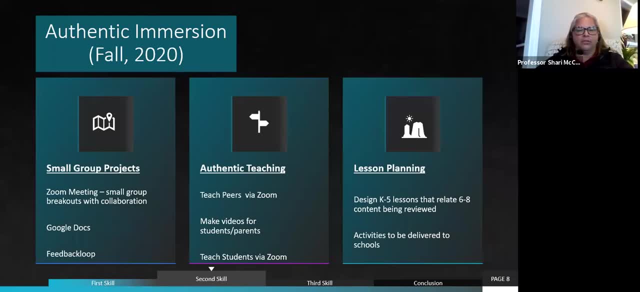 learning or simultaneous learning through learning or simultaneous learning through our class time, where they were not our class time, where they were not our class time, where they were not encouraging that for the spring. so we encouraging that for the spring, so we encouraging that for the spring. so we use, I use zoom and I use the small group. 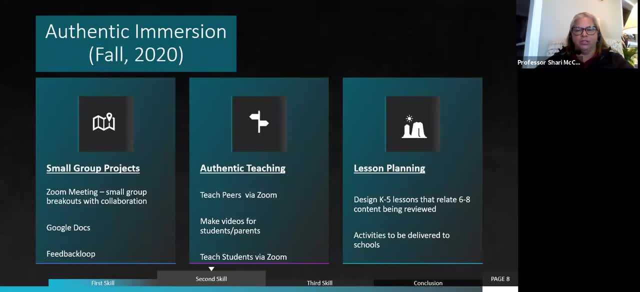 use- I use zoom and I use the small group use- I use zoom and I use the small group. breakout rooms for collaboration in breakout rooms, for collaboration in breakout rooms, for collaboration in which the students can use whiteboards which the students can use, whiteboards which the students can use, whiteboards share their screens, all sorts of things. 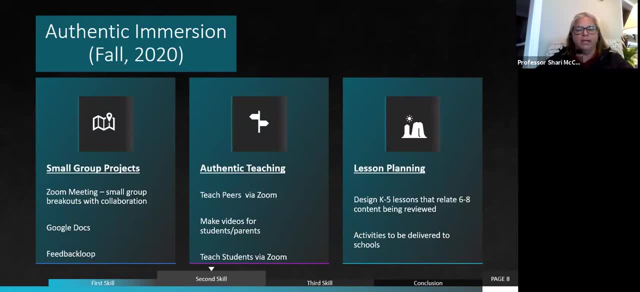 share their screens all sorts of things. share their screens, all sorts of things. that has worked wonderful because I can. that has worked wonderful because I can. that has worked wonderful because I can pop in and join the small breakout rooms. pop in and join the small breakout rooms. 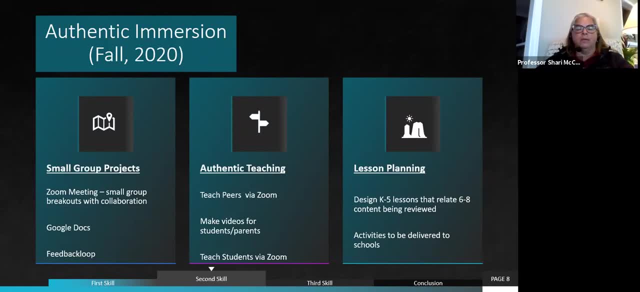 pop in and join the small breakout rooms and hear what they're saying. answer and hear what they're saying. answer and hear what they're saying. answer questions. call them back to the big group questions. call them back to the big group questions. call them back to the big group when I'm ready to reconvene things. 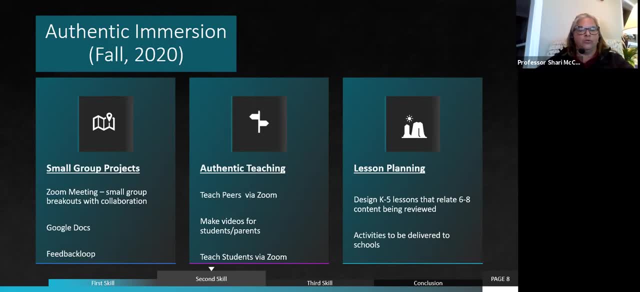 when I'm ready to reconvene things, when I'm ready to reconvene things like that. so I have really really enjoyed like that. so I have really, really enjoyed like that. so I have really really enjoyed the small group breakouts for our, the small group breakouts for our. 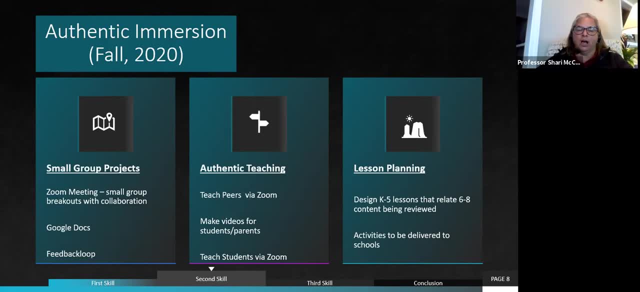 the small group breakouts for our projects. again, I oftentimes share a projects. again, I oftentimes share a projects. again. I oftentimes share a Google Doc with them so that they can Google Doc with them, so that they can Google Doc with them, so that they can make sure that their Google Doc is a. 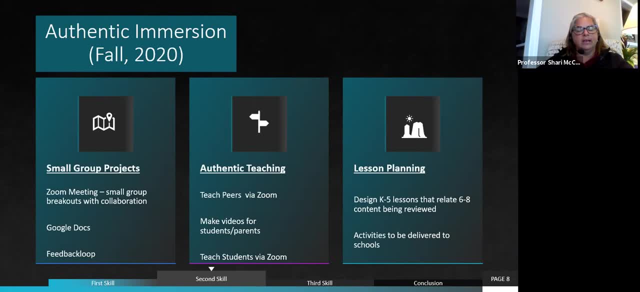 make sure that their Google Doc is a make sure that their Google Doc is a collaborative document happening, collaborative document happening. collaborative document happening simultaneously and the feedback loop is simultaneously and the feedback loop is simultaneously and the feedback loop is provided within the Google Doc, so our provided within the Google Doc, so our 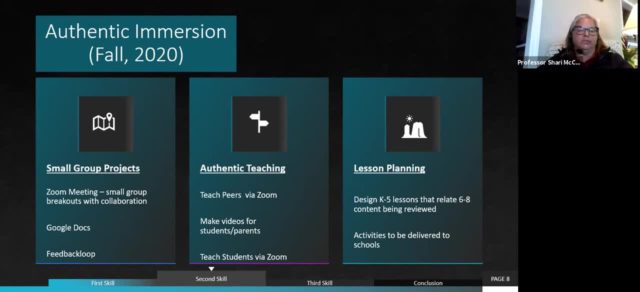 provided within the Google Doc. so our small projects really are being more small projects really are being more small projects really are being more productive- this fall with that breakout productive, this fall with that breakout productive, this fall with that breakout room within zoom. so I found that helpful. 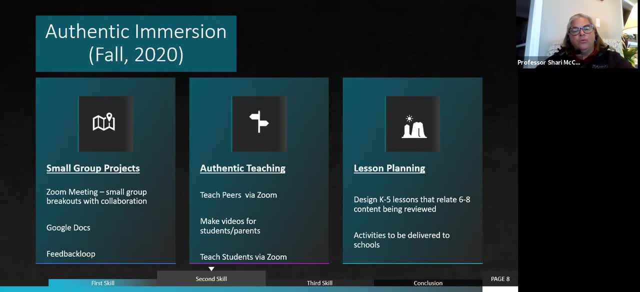 room within zoom, so I found that helpful. room within zoom, so I found that helpful. as for authentic teaching, we are hoping as for authentic teaching. we are hoping, as for authentic teaching. we are hoping to have our pre-service teachers teach, to have our pre-service teachers teach. 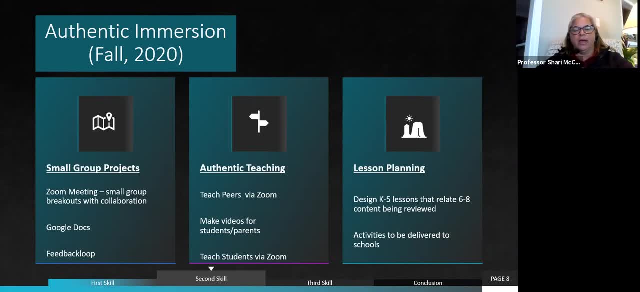 to have our pre-service teachers teach live via zoom into a classroom. third, live via zoom into a classroom. third, live via zoom into a classroom. third, fourth or fifth grade and they will work fourth or fifth grade and they will work fourth or fifth grade and they will work with small groups of students. so that is. 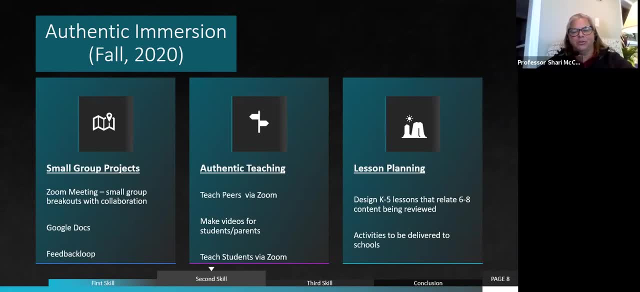 with small groups of students. so that is with small groups of students. so that is to start next month. so I'm not able to to start next month. so I'm not able to to start next month, so I'm not able to report exactly how that's going to work. 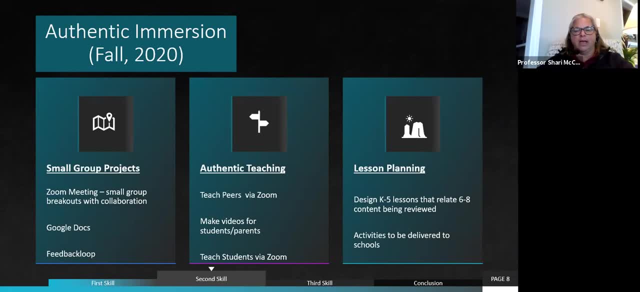 report exactly how that's going to work. report exactly how that's going to work. but we're super excited about the but we're super excited about the but we're super excited about the opportunity to once again see students, opportunity to once again see students, opportunity to once again see students in that grade band so that we can have 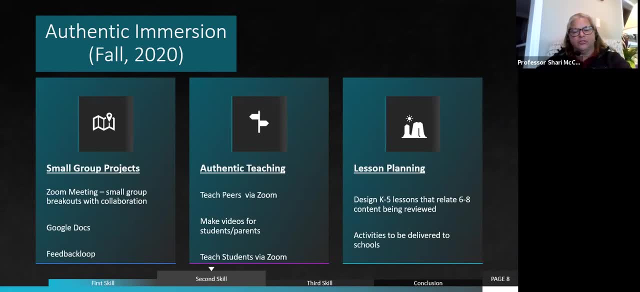 in that grade band so that we can have in that grade band, so that we can have much more of an authentic experience, much more of an authentic experience, much more of an authentic experience than volunteers and family members, that than volunteers and family members, that than volunteers and family members that we had in spring. once again, they'll. 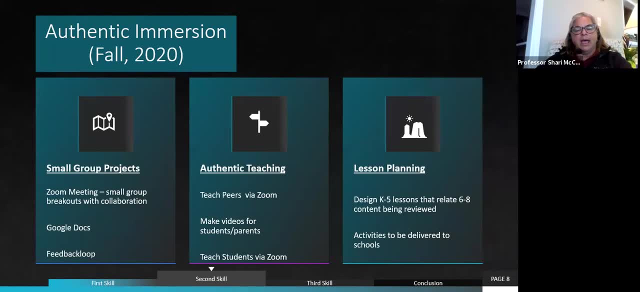 we had in spring. once again they'll we had in spring once again. they'll continue making videos for students and continue making videos for students and continue making videos for students and parents, and they will, they will teach parents and they will, they will teach parents and they will, they will teach their peers also using zoom. so the 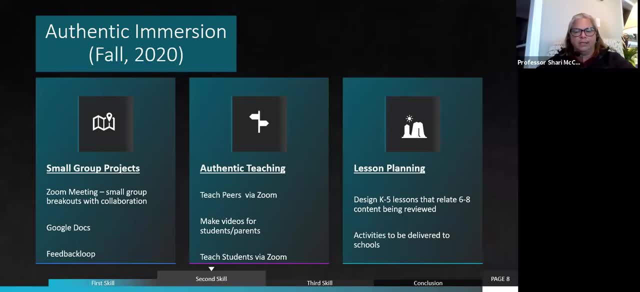 their peers also using zoom. so the their peers also using zoom. so the pre-service teachers will teach to their pre-service teachers will teach to their pre-service teachers will teach to their other Aquinas peers doing certain things. other Aquinas peers doing certain things, other Aquinas peers doing certain things. demonstrating methods that we have. 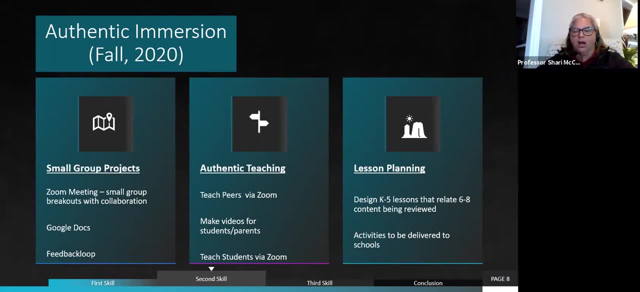 demonstrating methods that we have, demonstrating methods that we have learned. so we're using zoom fairly learned. so we're using zoom fairly learned. so we're using zoom fairly heavily this fall as a recommendation, heavily this fall as a recommendation, heavily this fall as a recommendation from the college, so that the students 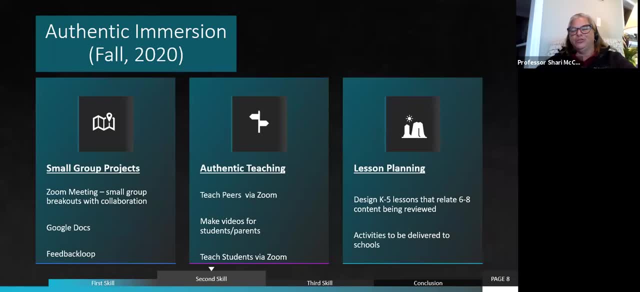 from the college so that the students from the college, so that the students can continue to use one or two platforms, can continue to use one or two platforms, can continue to use one or two platforms, instead of each professor picking their, instead of each professor picking their, instead of each professor picking their own. as far as lesson plans, we- I designed. 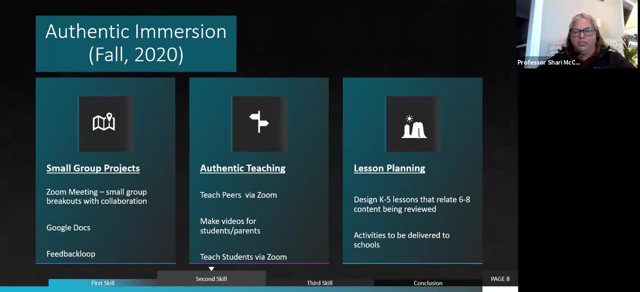 own as far as lesson plans we I designed. own as far as lesson plans we I designed something a little bit different. this something a little bit different. this something a little bit different. this semester, our math education content semester, our math education content semester, our math education content courses, resolve around a six through. 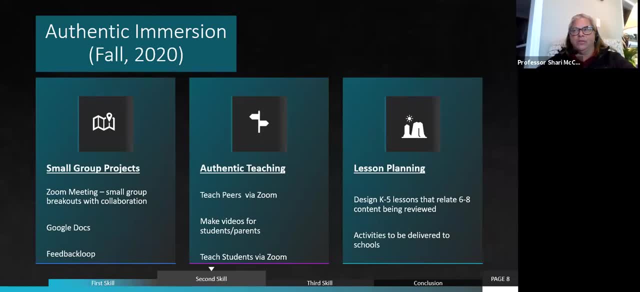 courses resolve around a six through courses resolve around a six through eighth math curriculum. and that's how eighth math curriculum and that's how eighth math curriculum and that's how they're reviewing their math content in they're reviewing their math content in. they're reviewing their math content in preparation of teaching K through five. 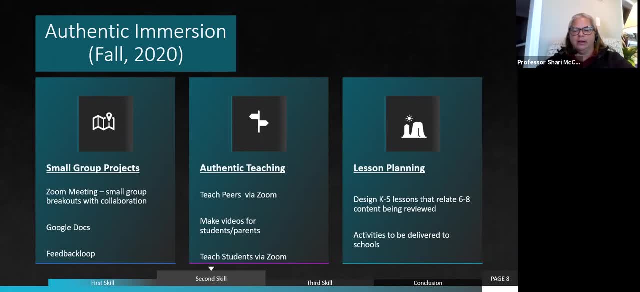 preparation of teaching K through five. preparation of teaching K through five. so as we review the six through eight, so as we review the six through eight, so as we review the six through eight content areas: they design lessons that content areas. they design lessons that content areas. they design lessons that would have been building foundations to. 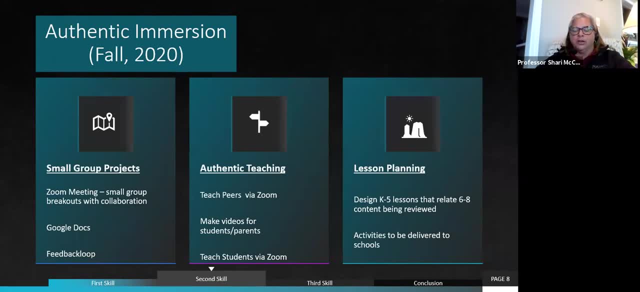 would have been building foundations to would have been building foundations to their own learning. so the Aquinas, their own learning. so the Aquinas their own learning. so the Aquinas student is building a lesson K through. student is building a lesson K through. student is building a lesson K through five. they get to pick and for example we: 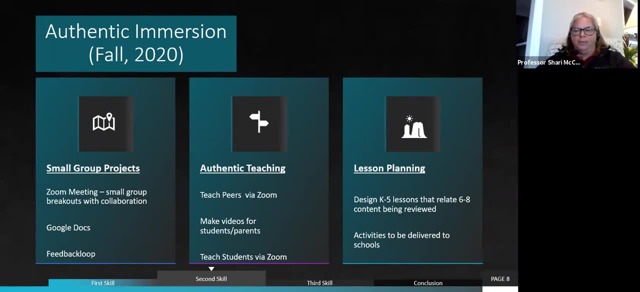 five they get to pick. and for example, we five, they get to pick. and for example, we just finished a linear algebra unit, so just finished a linear algebra unit, so just finished a linear algebra unit. so what topics K through five would support? what topics K through five would support? 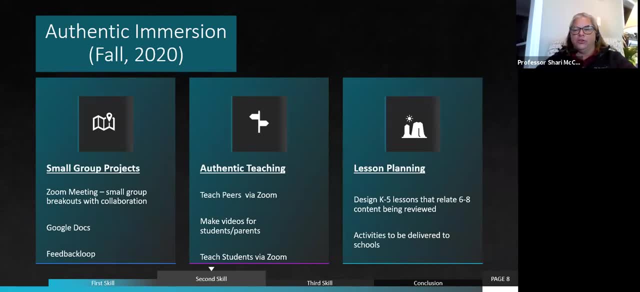 what topics K through five would support a linear algebra student in the future. a linear algebra student in the future. so someone picked patterning in. so someone picked patterning in. so someone picked patterning in kindergarten and how important it is to kindergarten and how important it is to 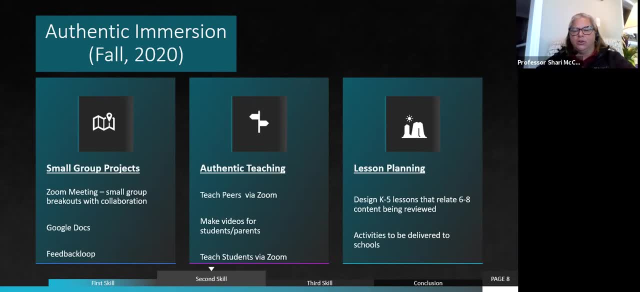 kindergarten and how important it is to understand patterns for algebra and so understand patterns for algebra and so understand patterns for algebra and so on. so this really helps the elementary on. so this really helps the elementary on. so this really helps the elementary teacher realize why it's important for 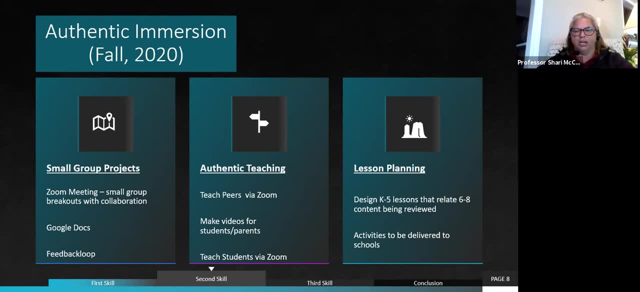 teacher realize why it's important for teacher, realize why it's important for them to have a strong content knowledge. them to have a strong content knowledge, them to have a strong content knowledge. above the grade they're teaching, but it. above the grade they're teaching, but it. 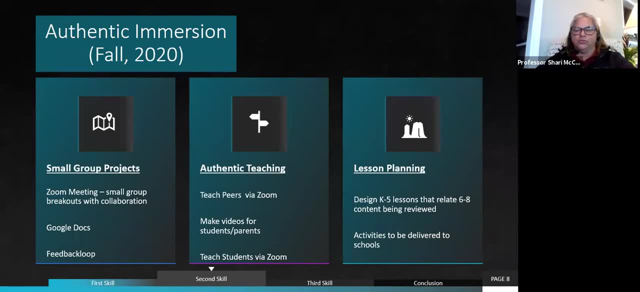 above the grade they're teaching, but it also should help them pick which things also should help them pick which things also should help them pick which things to stress in their own curriculum and to stress in their own curriculum and to stress in their own curriculum and classrooms- 3rd, 4th and 5th grade. so we 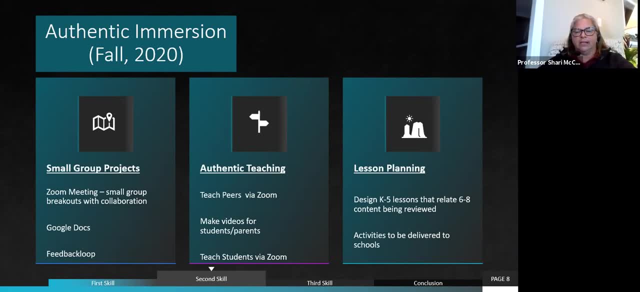 classrooms 3rd, 4th and 5th grade. so we classrooms 3rd, 4th and 5th grade. so we are designing and do this Wednesday the are designing and do this Wednesday. the are designing and do this Wednesday the activity that's hands-on, that we'll be. 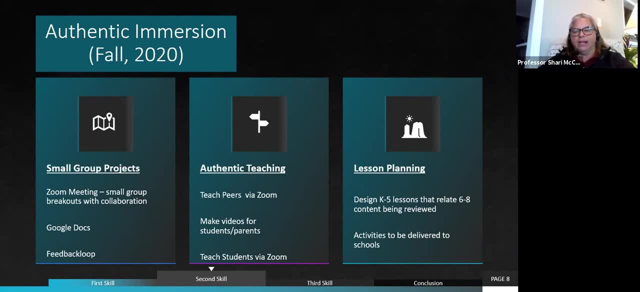 activity that's hands-on, that we'll be activity that's hands-on, that we'll be delivering in individual bags. so each delivering in individual bags, so each delivering in individual bags. so each student will receive an activity of student, will receive an activity of student, will receive an activity of their own and we'll be designing an. 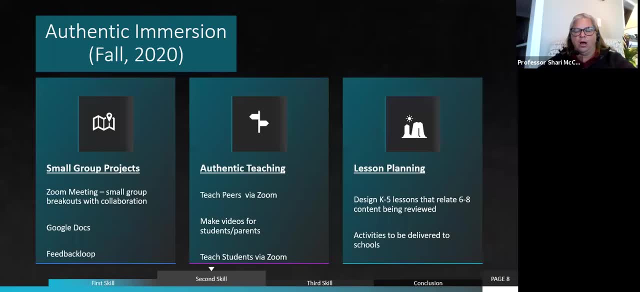 their own and we'll be designing an their own and we'll be designing an online activity for the student to do on online activity for the student to do on online activity for the student to do on their own online. we'll be designing an their own online activity for the student to do on their own online. we'll be designing an. 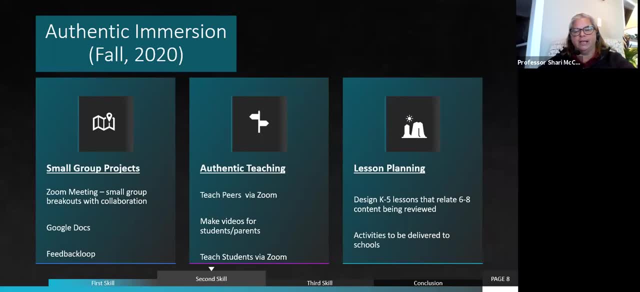 their own online activity for the student to do on their own online. we'll be designing an activity that the Aquinas students you do, activity that the Aquinas students you do. activity that the Aquinas students you do simultaneously online with the younger, simultaneously online with the younger. 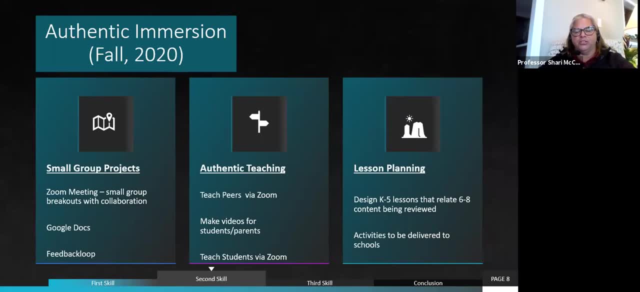 simultaneously online with the younger students, and then the last one will be a students, and then the last one will be a students, and then the last one will be a final project, will be an activity of final project, will be an activity of final project, will be an activity of their choice doing any of those three. 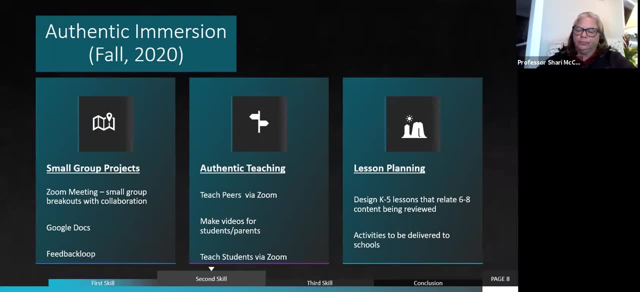 their choice: doing any of those three, their choice, doing any of those three formats for their students. so what formats for their students, so what formats for their students. so, what online tools did I use so I was able to? online tools did I use so I was able to. 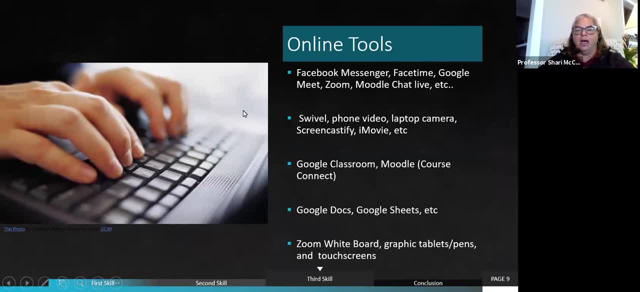 online tools did I use so I was able to use Facebook Messenger, FaceTime, Google. use Facebook Messenger, FaceTime, Google. use Facebook Messenger, FaceTime, Google, meet zoom. we use a Moodle chat platform- meet zoom. we use a Moodle chat platform- meet zoom. we use a Moodle chat platform at Aquinas so we had a chat live as far. 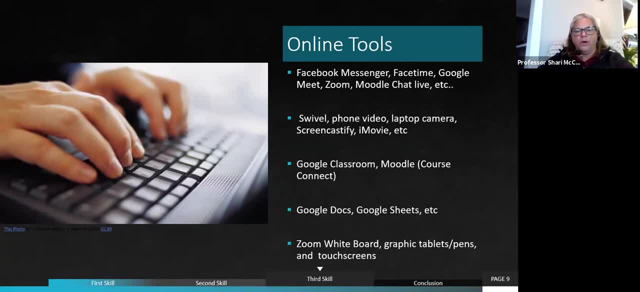 at Aquinas, so we had a chat live as far at Aquinas, so we had a chat live. as far as online technology hardware that we've as online technology hardware, that we've as online technology hardware that we've used- we use the swivel, if you're. 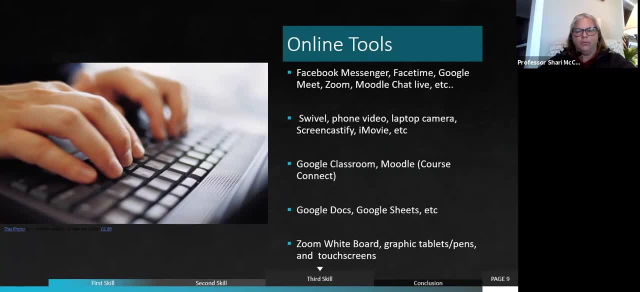 used, we use the swivel. if you're used, we use the swivel. if you're unfamiliar with the swivel, it's a unfamiliar with the swivel. it's a unfamiliar with the swivel. it's a lanyard that the teacher wears while an 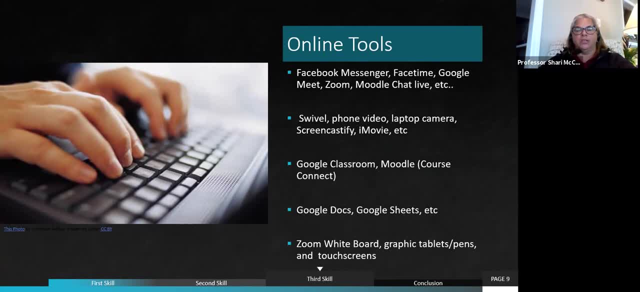 lanyard that the teacher wears, while an lanyard that the teacher wears, while an iPad or iPhone is hooked into the actual iPad or iPhone, is hooked into the actual iPad or iPhone, is hooked into the actual swivel. that way the camera follows you. swivel: that way the camera follows you. 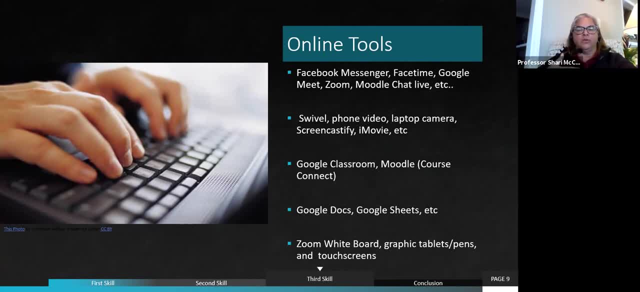 swivel. that way, the camera follows you where you walk around the classroom, the. where you walk around the classroom, the. where you walk around the classroom, the swivel moves your camera automatically. swivel moves your camera automatically. swivel moves your camera automatically for you, so you don't need someone. 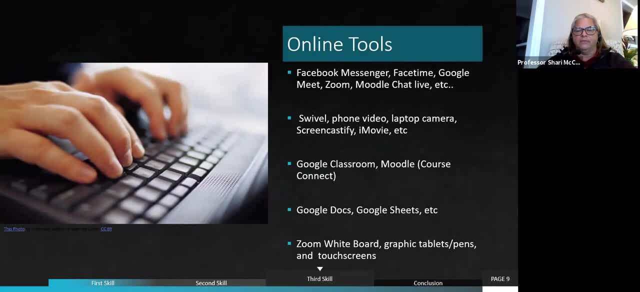 for you, so you don't need someone for you, so you don't need someone recording. yet you're always the center recording. yet you're always the center recording, yet you're always the center of the of the video and the swivel of the of the video and the swivel. 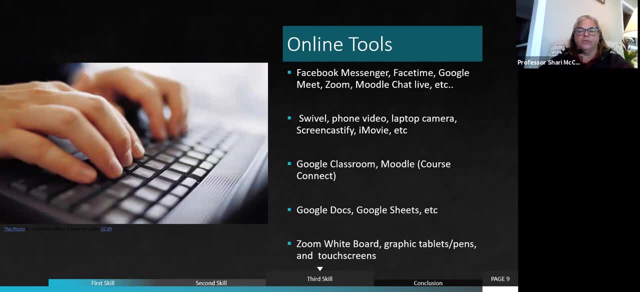 of the of the video and the swivel lanyard has a microphone. so that if you lanyard has a microphone, so that if you lanyard has a microphone, so that if you turn your back to the swivel your mic, turn your back to the swivel your mic. 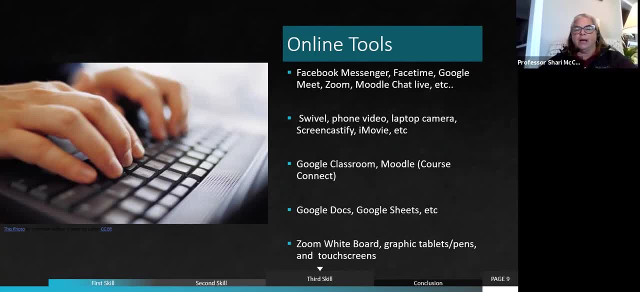 turn your back to the swivel. your mic, your microphone still sounds great. we've your microphone still sounds great. we've your microphone still sounds great. we've used laptop cameras. we've caught our used laptop cameras. we've caught our used laptop cameras. we've caught our screens and screencastify so that, as 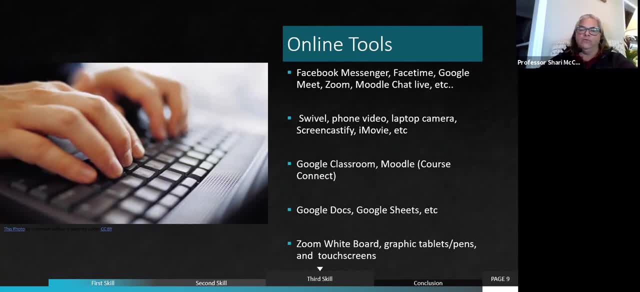 screens and screencastify so that as screens and screencastify, so that, as we're doing something, it's creating a, we're doing something. it's creating a we're doing something, it's creating a video. iMovie, all of those types of video. iMovie, all of those types of. 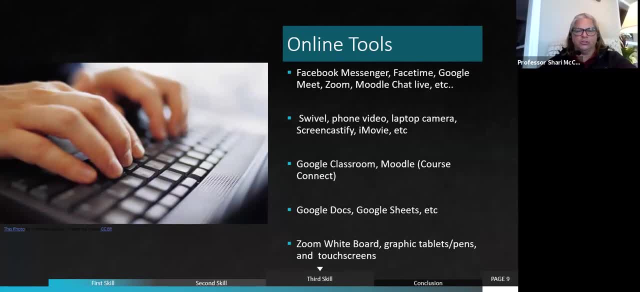 video, iMovie, all of those types of things would be some of the online tools. things would be some of the online tools. things would be some of the online tools. so I tried not to restrict my students, so I tried not to restrict my students, so I tried not to restrict my students in what they used, and I also tried to 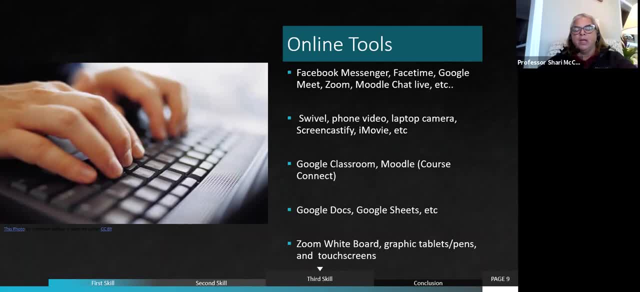 in what they used and I also tried to in what they used and I also tried to use a wide variety for them to see how. use a wide variety for them, to see how. use a wide variety for them to see how that would work. our content was: 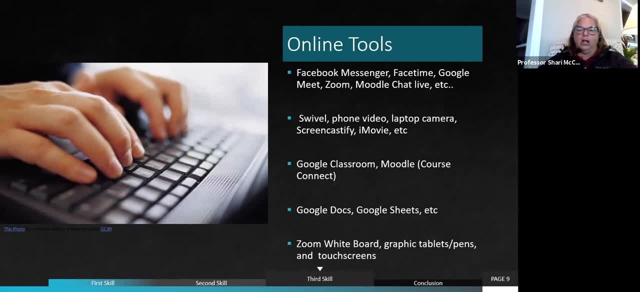 that would work. our content was that would work. our content was primarily in Google classroom and at the, primarily in Google classroom and at the, primarily in Google classroom and at the college were required to use what we college were required to use, what we college were required to use what we call Aquinas course connect, which I 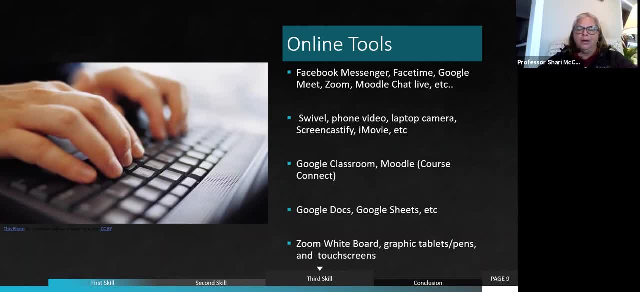 call Aquinas course connect, which I call Aquinas course connect, which I mentioned was a Moodle based platform. I mentioned was a Moodle based platform. I mentioned was a Moodle based platform. I already discussed, discussed my love for already discussed. discussed my love for already discussed. discussed my love for Google Docs and simultaneous. 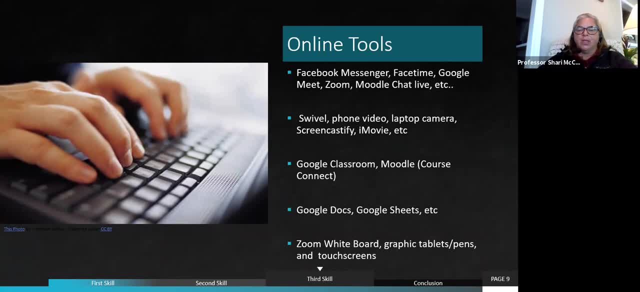 Google Docs and simultaneous Google Docs and simultaneous contributions. we also did Google sheets contributions. we also did Google sheets contributions. we also did Google sheets within zoom. we've used the whiteboard within zoom. we've used the whiteboard within zoom. we've used the whiteboard application- both myself and also the. 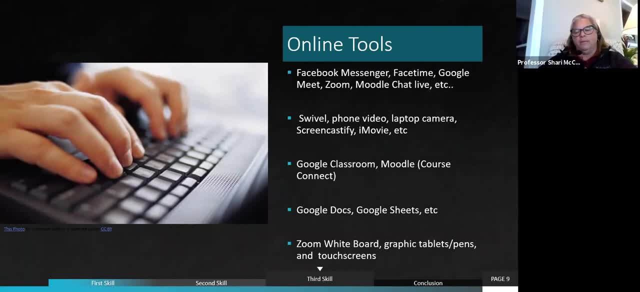 application, both myself and also the application, both myself and also the students. I've used a graphic tablet pen students. I've used a graphic tablet pen students. I've used a graphic tablet pen and some of my students have touch and some of my students have touch and some of my students have touch screens that they were able to share. 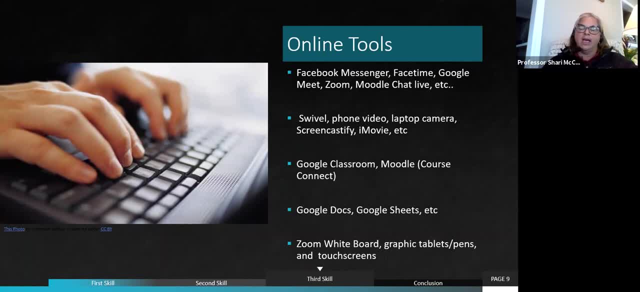 screens that they were able to share, screens that they were able to share with. so we've used a wide variety in the with. so we've used a wide variety in the with. so we've used a wide variety in the last six months, and I'm gonna talk to. 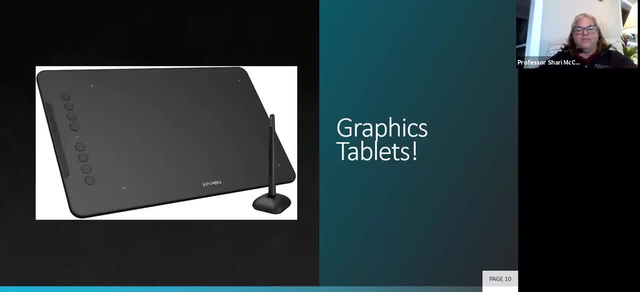 last six months and I'm gonna talk to last six months and I'm gonna talk to you a little bit about some of my you, a little bit about some of my you, a little bit about some of my favorites. so one of my favorites is this favorites. so one of my favorites is this: 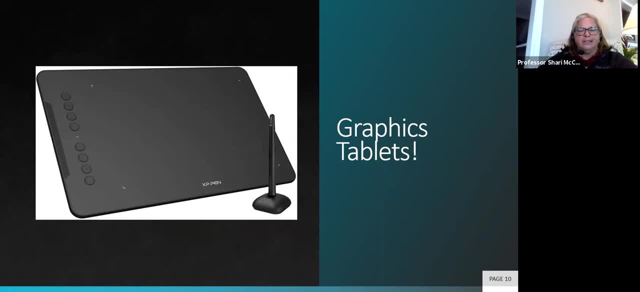 favorites. so one of my favorites is this graphic tablet. some people call it a graphic tablet, some people call it a graphic tablet, some people call it a graphic pen. it's simply this black piece graphic pen. it's simply this black piece graphic pen. it's simply this black piece. it almost is like a clipboard and it. 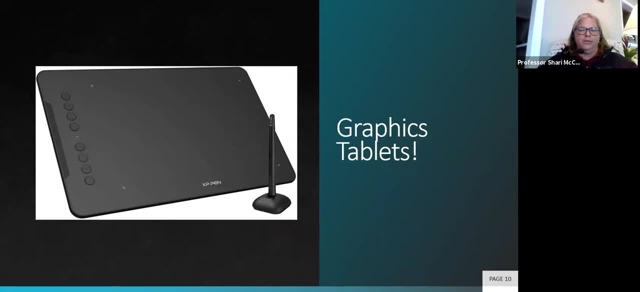 it almost is like a clipboard and it it almost is like a clipboard and it comes with a pen and you draw on the comes with a pen and you draw on the comes with a pen and you draw on the blackboard which you don't see anything. 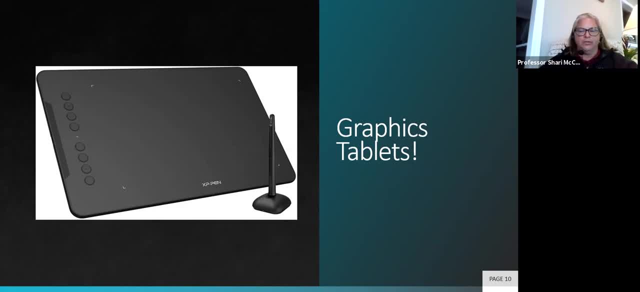 blackboard which you don't see anything. blackboard which you don't see anything is very involved. if you need to upload is very involved. if you need to upload is very involved if you need to upload drivers or things in your individual. drivers or things in your individual. 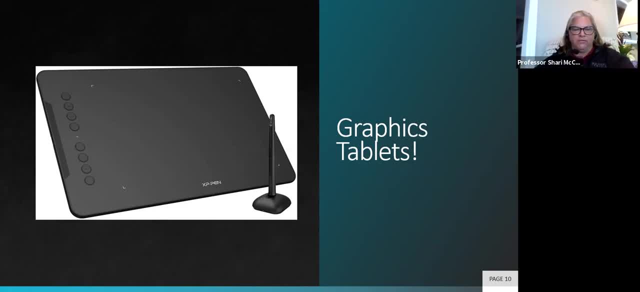 drivers or things in your individual classrooms. it becomes really cumbersome classrooms. it becomes really cumbersome classrooms. it becomes really cumbersome for the college professor because we do for the college professor, because we do for the college professor, because we do not teach in the same classroom at our, not teach in the same classroom at our. 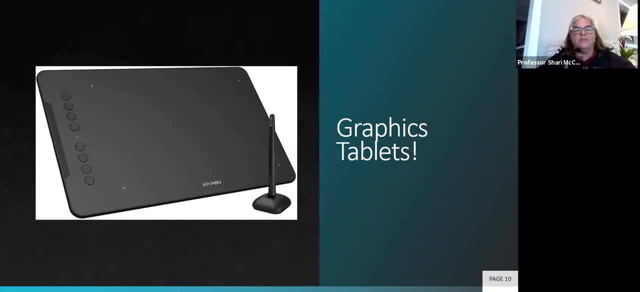 not teach in the same classroom at our institution. so I couldn't couldn't have institution. so I couldn't couldn't have institution, so I couldn't couldn't have them upload a few drivers. they would have them upload a few drivers. they would have them upload a few drivers. they would have been against it, but this graphic tablet. 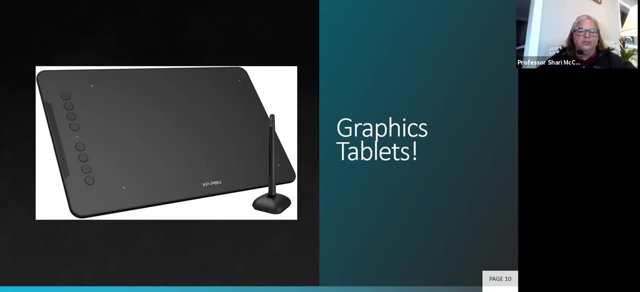 been against it. but this graphic tablet been against it. but this graphic tablet is simply a USB plug and it's ready to go- is simply a USB plug and it's ready to go. is simply a USB plug and it's ready to go. so it's wonderful. every computer, I stop. 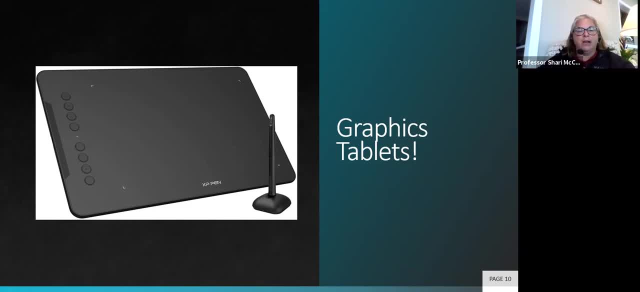 so it's wonderful. every computer, I stop. so it's wonderful. every computer, I stop it. I just plug it in and my pen is ready it. I just plug it in and my pen is ready it. I just plug it in and my pen is ready to go. the pen also acts as a mouse, so 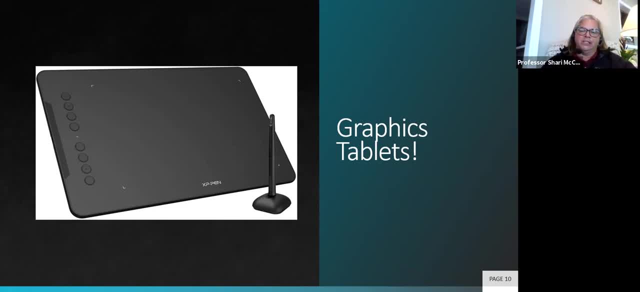 to go, the pen also acts as a mouse. so to go, the pen also acts as a mouse. so you'll know exactly what's happening. you'll know exactly what's happening. you'll know exactly what's happening because you'll see the light, so for. because you'll see the light, so for. 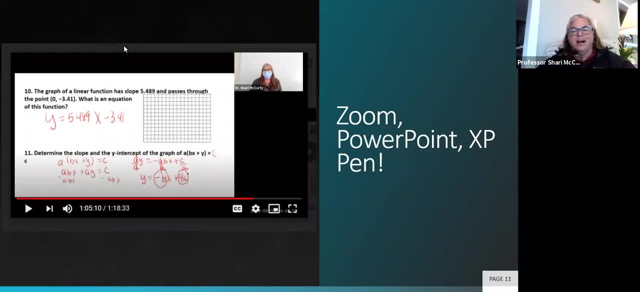 because you'll see the light. so, for example, yes, this is me with my mask on example. yes, this is me with my mask on example, yes, this is me with my mask on because one of my classes I teach half, because one of my classes I teach half. 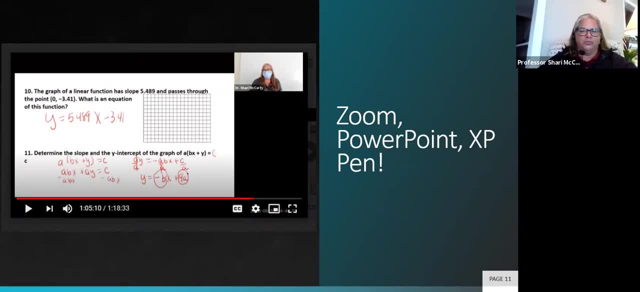 because one of my classes I teach half of the class in face-to-face, while the of the class in face-to-face, while the of the class in face-to-face, while the other half watches in zoom, that's on. other half watches in zoom, that's on. 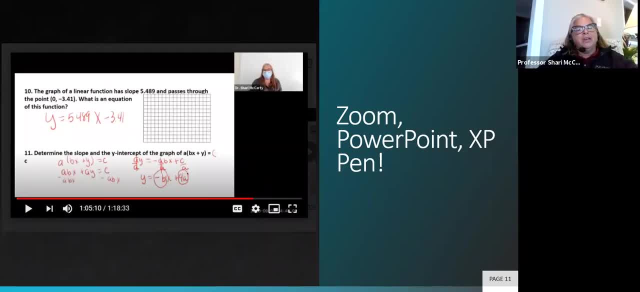 other half watches in zoom. that's on Monday, and then they reverse roles on Monday, and then they reverse roles on Monday, and then they reverse roles on Thursday. so I typically do a PowerPoint Thursday. so I typically do a PowerPoint Thursday. so I typically do a PowerPoint with some problems, and then I use my 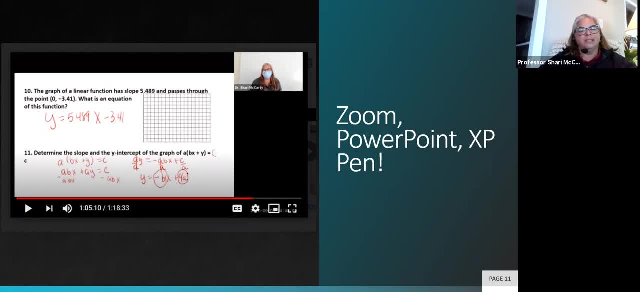 with some problems, and then I use my with some problems, and then I use my graphic tablet to write over my graphic tablet, to write over my graphic tablet, to write over my PowerPoint. and this is what it would PowerPoint, and this is what it would PowerPoint, and this is what it would look like and it's captured live during. 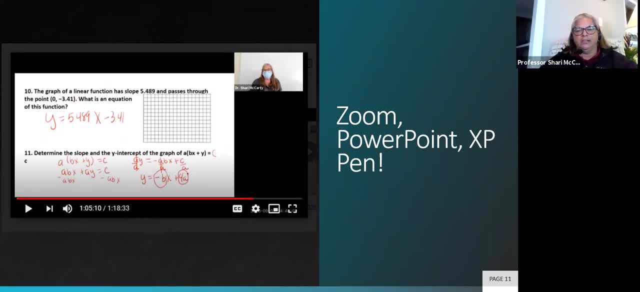 look like and it's captured live during: look like and it's captured live during my zoom recording so that students can my zoom recording, so that students can my zoom recording, so that students can actually see me working in real time- if, actually see me working in real time, if. 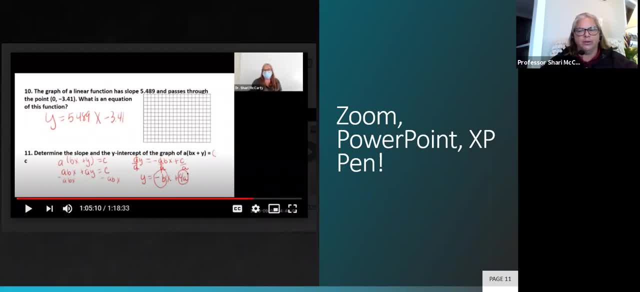 actually see me working in real time. if they go back and watch the video. if they go back and watch the video. if they go back and watch the video if they're absent due to kovat or any other. they're absent due to kovat or any other. 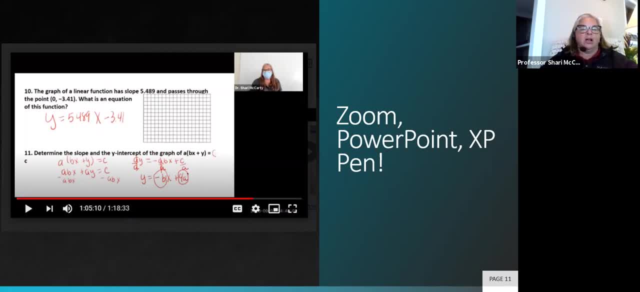 they're absent due to kovat or any other absence. so you can change obviously the absence. so you can change obviously the absence, so you can change obviously the color of the pen or the ink that shows color of the pen or the ink that shows color of the pen or the ink that shows up. but it's very, very simple to use. I. 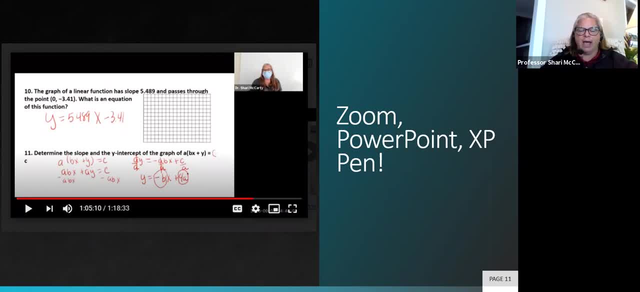 up, but it's very, very simple to use. I up, but it's very, very simple to use. I have literally got this pen about two. have literally got this pen about two. have literally got this pen about two and a half weeks ago and I'm super. and a half weeks ago and I'm super. 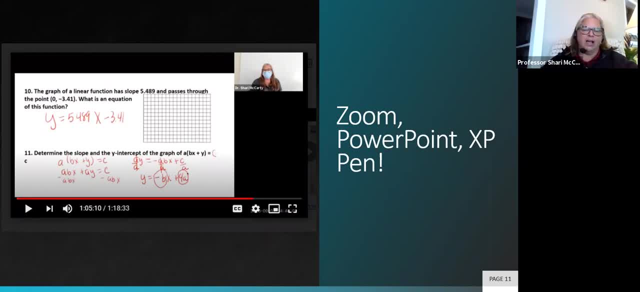 and a half weeks ago and I'm super comfortable with it and anyone could use comfortable with it and anyone could use comfortable with it and anyone could use it. so I highly encourage this. this is a it. so I highly encourage this. this is a it, so I highly encourage this. this is a cheap take. they run between 40 and 90. cheap take. they run between 40 and 90 cheap take. they run between 40 and 90 dollars. mine happened to be 60- it was dollars. mine happened to be 60- it was dollars. mine happened to be 60. it was kind of middle of the road and it does. 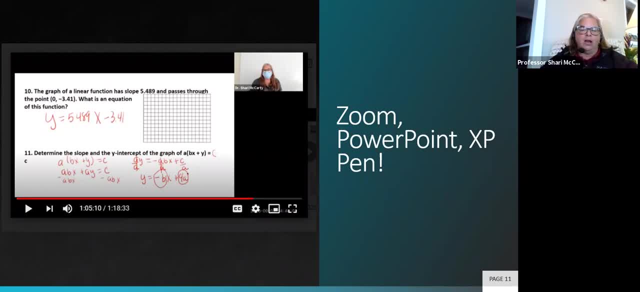 kind of middle of the road, and it does kind of middle of the road and it does everything that I'd like it to before I, everything that I'd like it to before I, everything that I'd like it to before I move on. I want to just stop about this. 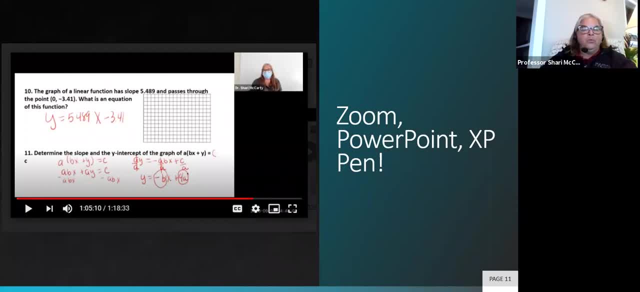 move on. I want to just stop about this, move on. I want to just stop about this whole PowerPoint zoom record pen. one of whole PowerPoint zoom record pen. one of whole PowerPoint zoom record pen. one of the really nice things about doing this. the really nice things about doing this. 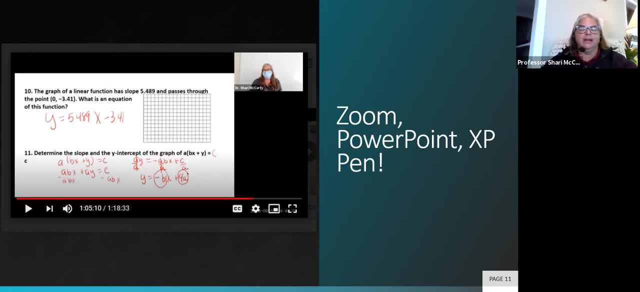 the really nice things about doing this. so I'm teaching live to my class, so I, so I'm teaching live to my class, so I, so I'm teaching live to my class. so I see the faces. it helps me have the. see the faces, it helps me have the. 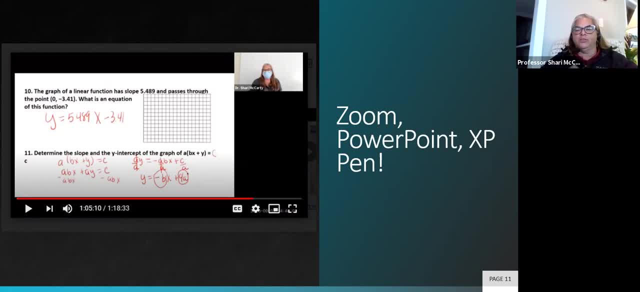 see the faces. it helps me have the expressions and know what to write and expressions and know what to write and expressions and know what to write and where their questions are, but at the where their questions are, but at the where their questions are. but at the same time, my zoom family is watching in. 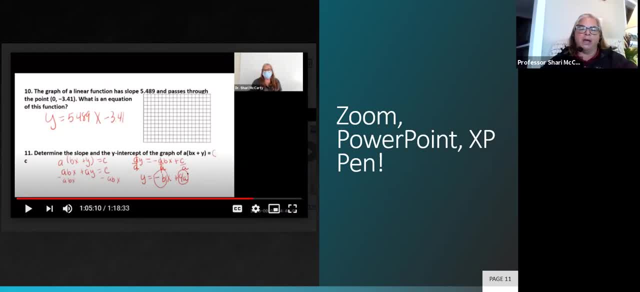 same time. my zoom family is watching. in same time, my zoom family is watching in live time and they're able to see this live time and they're able to see this live time and they're able to see this much better than they do. the whiteboard. 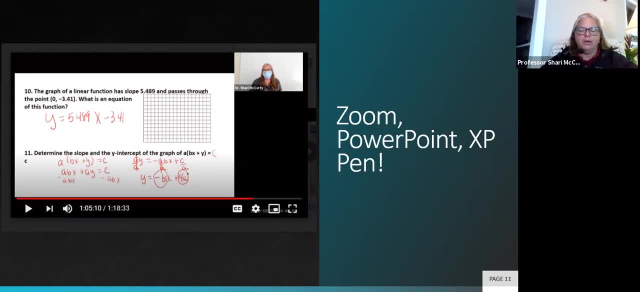 much better than they do the whiteboard, much better than they do the whiteboard behind me in our institution, the webcam behind me in our institution, the webcam behind me in our institution. the webcam is located on a fixed PC in the is located on a fixed PC in the. 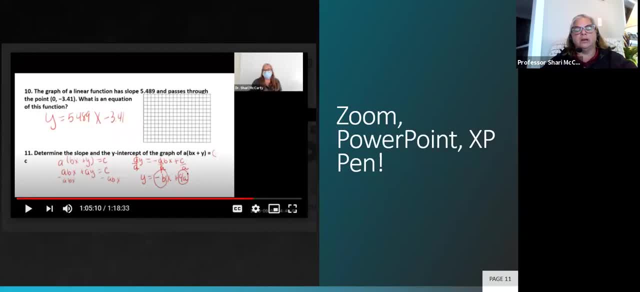 is located on a fixed PC in the classroom, so it only zooms of that classroom. so it only zooms of that classroom. so it only zooms of that picture. that you see of me in the upper picture, that you see of me in the upper picture, that you see of me in the upper right, is simply the amount of whiteboard. 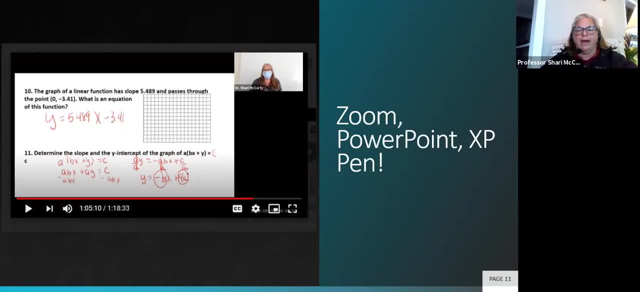 right is simply the amount of whiteboard. right is simply the amount of whiteboard behind me that the camera would capture behind me, that the camera would capture behind me, that the camera would capture. so between that and reflections of, and so between that and reflections of, and. 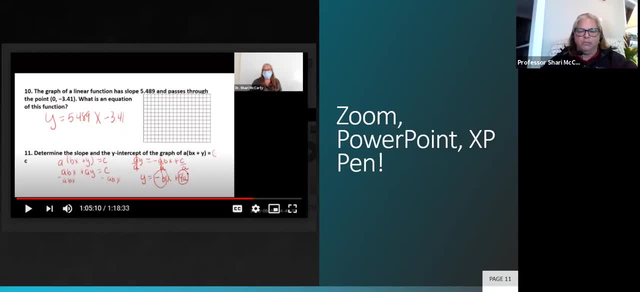 so between that and reflections of and running out of dark ink in your Expo, running out of dark ink in your Expo, running out of dark ink in your Expo markers, I really found that just writing markers. I really found that just writing markers. I really found that just writing over the PowerPoint. it really works. 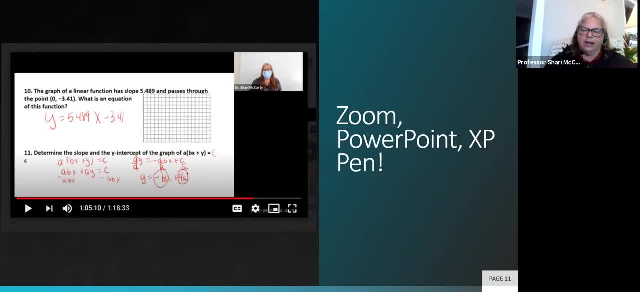 over the PowerPoint. it really works over the PowerPoint. it really works better than any other screen capture. any better than any other screen capture, any better than any other screen capture. any other idea that I've done super easy. other idea that I've done super easy. other idea that I've done super easy: super fast. zoom allows you to upload. 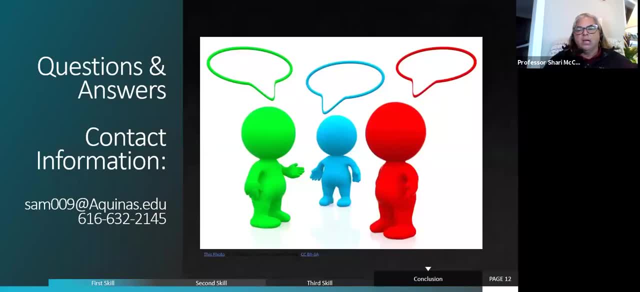 super fast zoom allows you to upload. super fast zoom allows you to upload your videos for sharing so with that and your videos for sharing so with that and your videos for sharing so with that. and I said my presentation would take about. I said my presentation would take about. 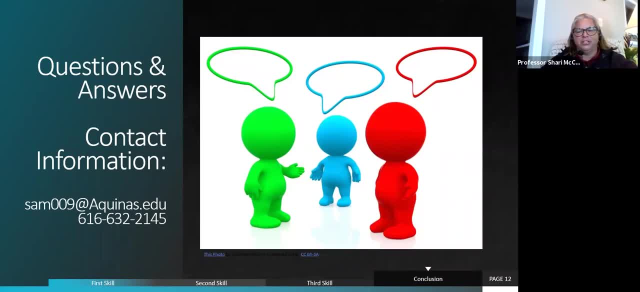 I said my presentation would take about 25 minutes and I'm a little bit ahead by 25 minutes and I'm a little bit ahead by 25 minutes and I'm a little bit ahead by a minute or two, but I do want to remind a minute or two, but I do want to remind. 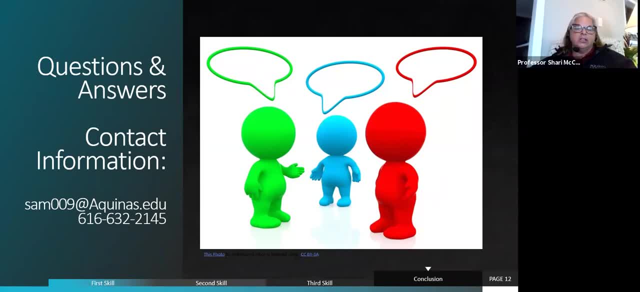 a minute or two, but I do want to remind you, before we open it up for question you, before we open it up for question you, before we open it up for question and answers, to write down the contact and answers. to write down the contact and answers. to write down the contact information, if you feel like you would. 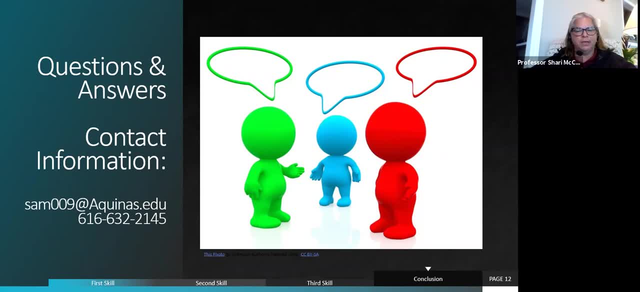 information if you feel like you would information if you feel like you would like to reach out and brainstorm, or hear like to reach out and brainstorm, or hear like to reach out and brainstorm, or hear more about what I'm doing? share what? more about what I'm doing? share what. 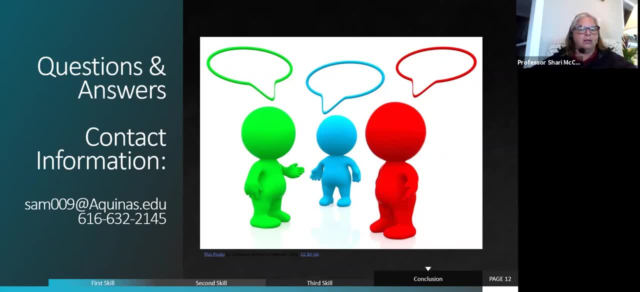 more about what I'm doing, share what you're doing, or you simply can call so you're doing, or you simply can call so you're doing, or you simply can call so. the email is S a m 0 0, 9 at Aquinas. the email is S a m 0 0, 9 at Aquinas.